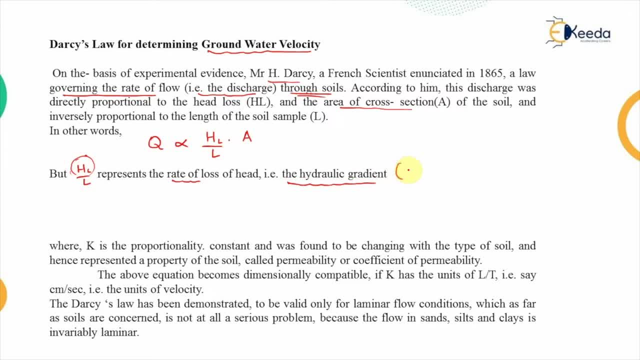 This is known as the hydraulic gradient, which is denoted by symbol I. So in place of HL upon L, we can replace this by I into A. Now, if we remove this proportionality sign, we get a constant value, that is, K into I into A. 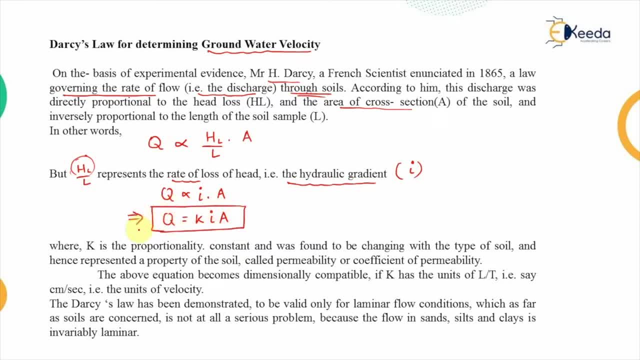 Now this is the formulation given by the Darcy's, Where K is a proportionality constant and when we experimented and the data was collected regarding the different type of soil, it was found to be changing with the type of soil and therefore it was represented as the property of a soil. 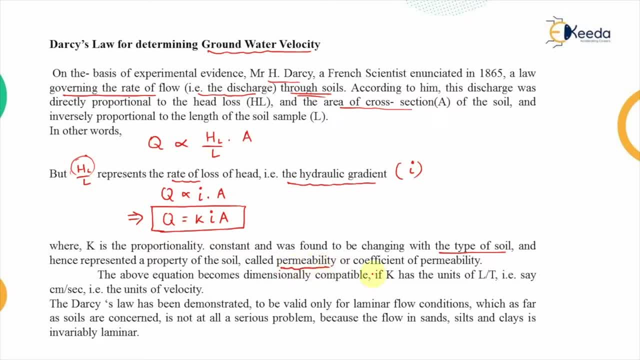 And that property is known as the permeability or the coefficient of permeability. Now this equation becomes dimensional. It is not necessarily compatible, because we know this: Q is the rate of flow, that is, cubic meter per second. For the K, we do not know the units. 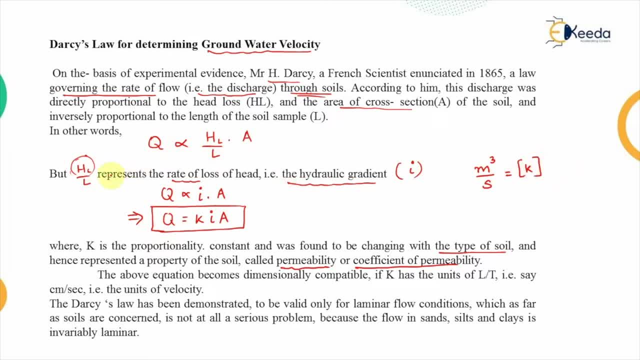 For hydraulic gradient. this is length upon length, So it will be unit less into the unit of area is square meter. So if we cancel this out, So the unit of this permeability, that is meter per second. So the above equation becomes dimensionally compatible if this permeability has the units of length per unit time. 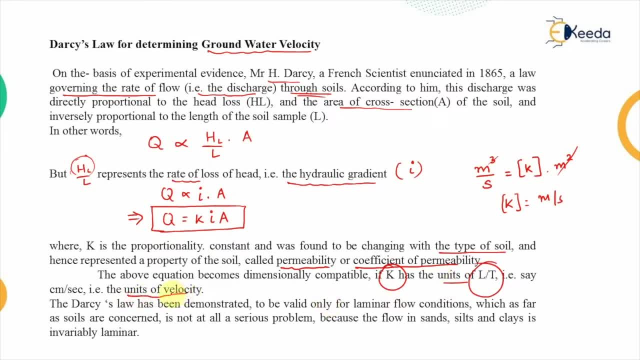 That is, the units of the velocity. The Darcy's law. This was demonstrated to be valid only for laminar flow conditions. That means, when the flow is taking place in such a way That there are adjacent levels, That there are adjacent levels. 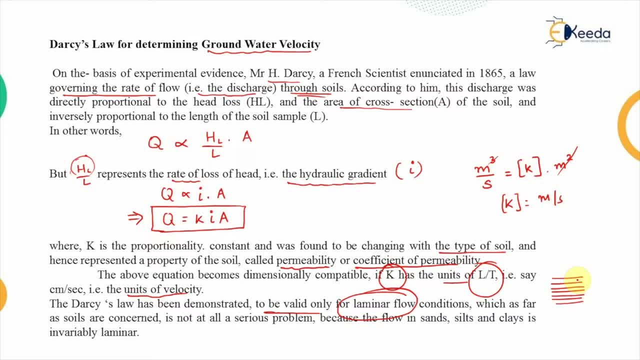 That there are adjacent levels, laminar, which are flowing one over the other, which, in case of soil, is not at all a serious problem, because the flow in sands, silt or the clay that is invariably laminar. We do not need to make the flow to be laminar Now from the previous equation, that is, Q is: 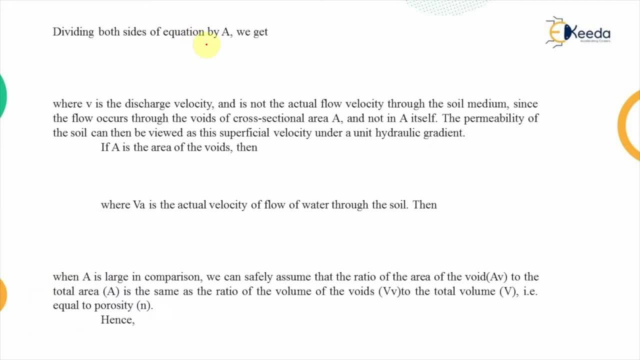 equal to kia. if we divide both the sides of the equation by the area, it will be: Q upon a is equal to k into ia divided by a. So this a will be cancelled out. Now from here, this Q upon a, that is, discharge upon area, that is known as the velocity and that is, is equal to k into i. 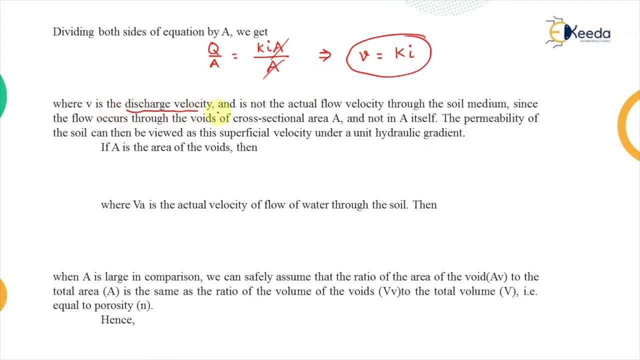 Now where V is the discharge velocity and is not the actual flow velocity through the soil medium. and the difference between this discharge velocity and the actual flow velocity is that this discharge is taking place through the voids of the cross-sectional area and not the area total area in itself. because of this, this is considered to be the 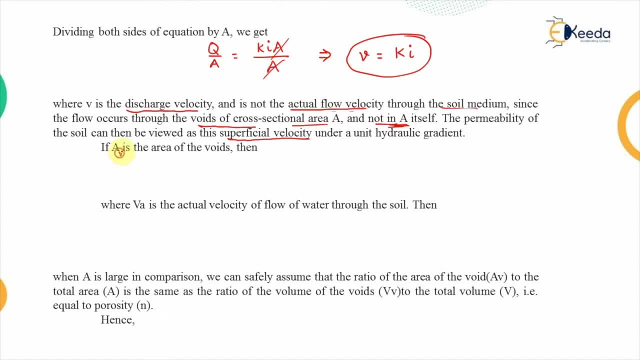 velocity. Now, if we consider the area of voids to be AV, then in that case the area of voids that is multiplied by the actual velocity that is taking place through the voids will be equal to the total area into this superficial velocity, where VEA is the actual velocity of the flow. 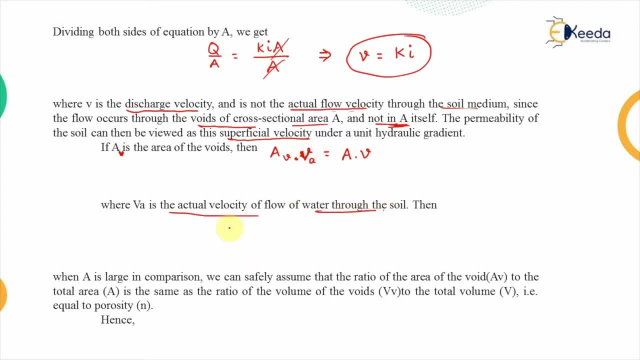 through the soil, Then VEA will be calculated as VA into AV upon A. Now, if the area of the medium is large in comparison to the area of the voids, we can safely assume that this ratio of AV upon A, that is same as volume of voids to the total volume, and this is nothing but the porosity. 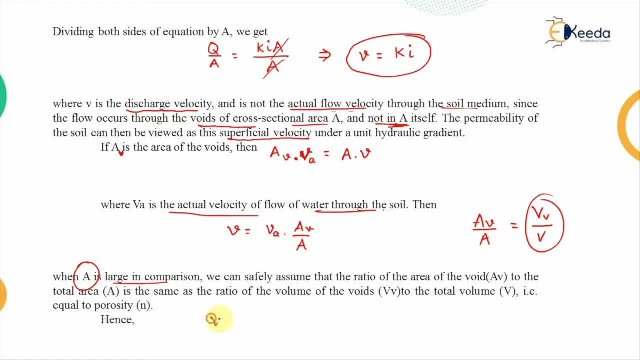 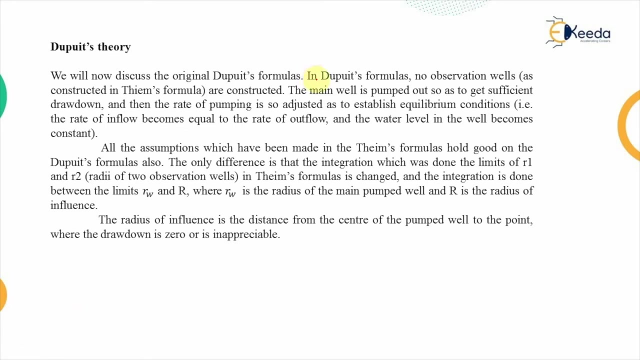 interval. Therefore the flow velocity or the discharge velocity that is equal to the actual velocity into the porosity, Therefore the discharge velocity is lesser than the actual velocity. So that completes the discussion regarding the Darcy's law. Now, next is Dupuit's theory. So this Dupuit's theory was originally considered and it was the 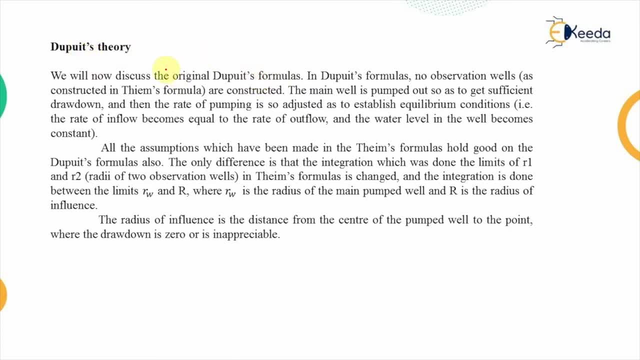 out of Dupitz and the Themes theory. However, we usually discuss the Themes theory first and then the discussion of Dupitz theory is carried out After studying the Themes theory. it is bit easier to study about the Dupitz In Dupitz. what are the changes than the Themes? First change is that? no observation. 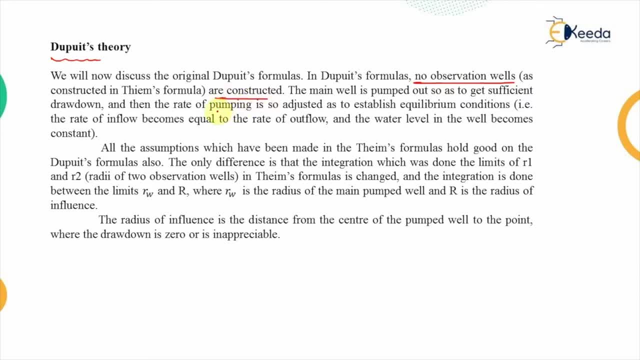 well is constructed. in case of the Dupitz theory, as was in the case of Themes formula, The main well is pumped out so as to get the sufficient drawdown, and then the rate of pumping is so adjusted so as to establish the equilibrium condition, ie the steady state is achieved, ie the rate. 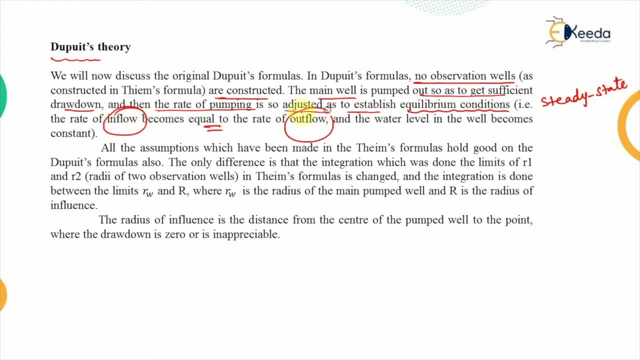 of inflow that becomes equal to the rate of outflow, and if this happens, then water level in the well that becomes constant. Now all the assumptions which we have made in the Themes theory that hold true in Dupitz theory also. the only difference here will be that instead of the limits, 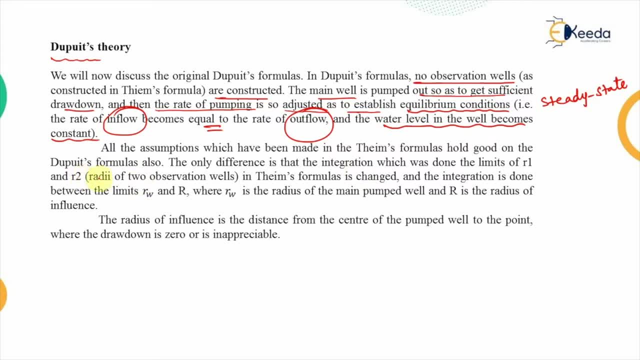 which we used in the Themes theory ie, R1 and R2, which were the radiuses of the two observation wells. here we will be integrating it in the range of Rw to R, where Rw is the radius of the main pumped well And R is the radius of the influence. Now, what is this radius of influence? It is: 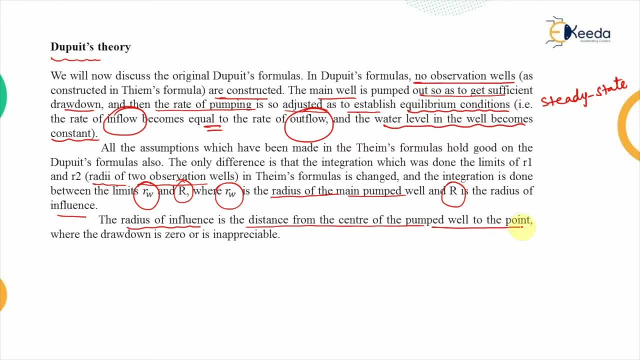 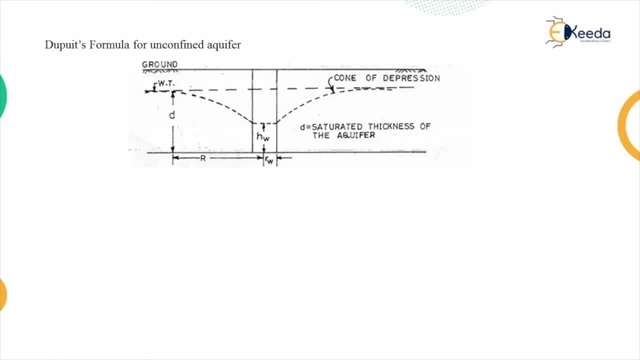 the distance from the center of the pumped well to the point where the drawdown is zero or isn't appreciable. That means where the drawdown has completely been eliminated. Now we know that we are having two types of aquifer. One is the. 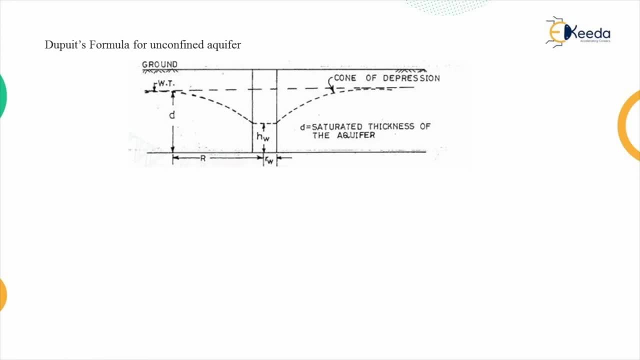 unconfined aquifer and other one is the confined aquifer. So, one by one, what are the formulas given by the Dupitz that we are going to discuss Now? Dupitz formula for the unconfined aquifer. So here there is only one impervious strata and the top 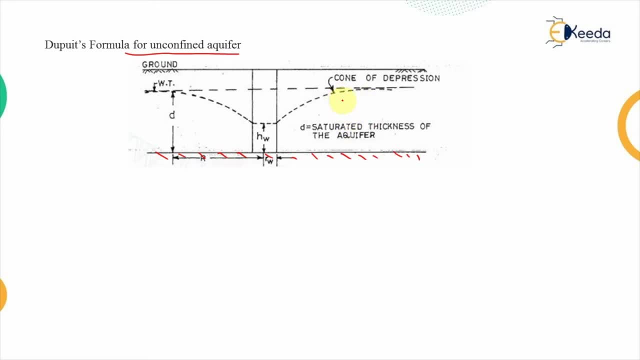 layer is free. Therefore, we can easily extract the water out of this. As we start extracting the water out of it, the water level drops down To this Hw level and the same profile is managed up to the last point of the drawdown. 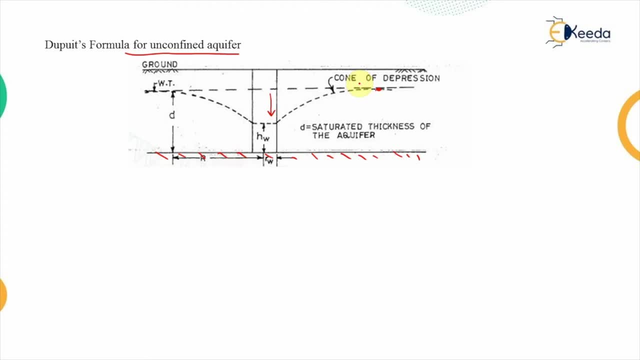 So this shape which is assumed, that is known as the cone of depression. Now we know that this discharge is equal to K, x, I, x, A, where I is the hydraulic gradient. So if we consider a small section, So for that the height of the water level, that is dH for length of dr Area of this. 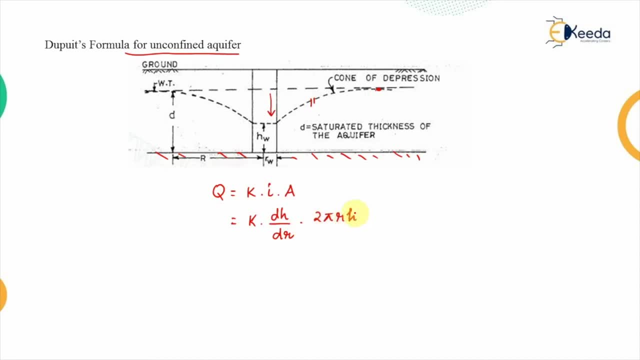 cylinder. that is 2 pi rh. Here K is the coefficient of permeability. Now, if we rearrange the terms, this will be dr upon r, that is equal to 2 pi. K upon q, into h, into dH. We have to integrate this into dH. 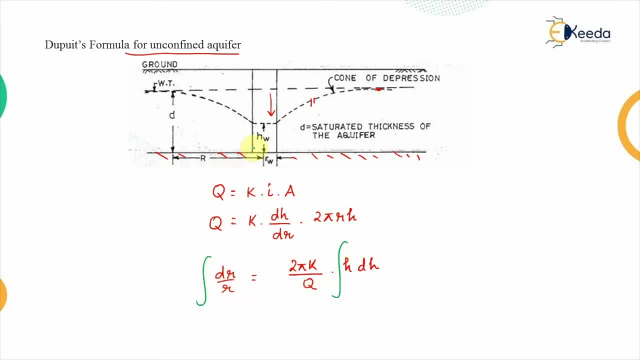 equation. so the radius will be varying for the main well- this is the main well- having the radius Rw, and this is the point where the influence zone is eliminated. so this radius is known as the radius of influence, denoted by capital R. so the limits will be Rw to R for the level of water from Hw to the. 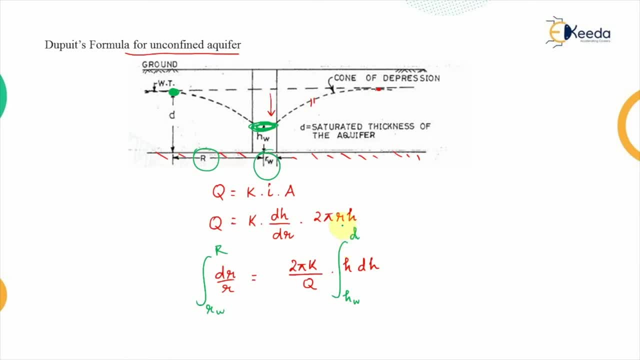 complete level, that is d. so if we integrate this, what we are getting as the natural log of R. now limits for this are from Rw to capital R, then 2 pi k upon Q. this is H square by 2. limits are written as equal to the size of the entire high point of the base. so this: 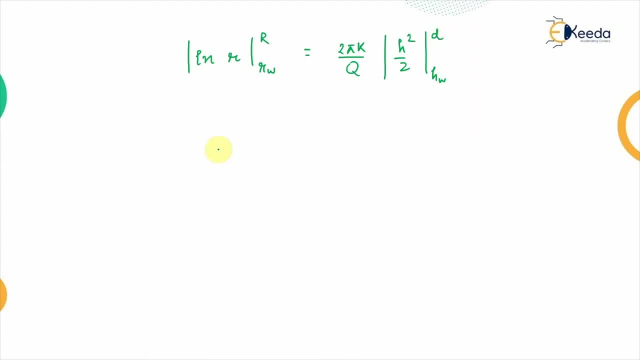 from hw to d. So this will be natural. log capital R upon rw is equal to this. 2 will be cancelling out the other 2.. So it will be pi k upon q limits from d square minus hw square. Therefore the rate of flow, if we summarize it, it will be pi k into d square minus hw. 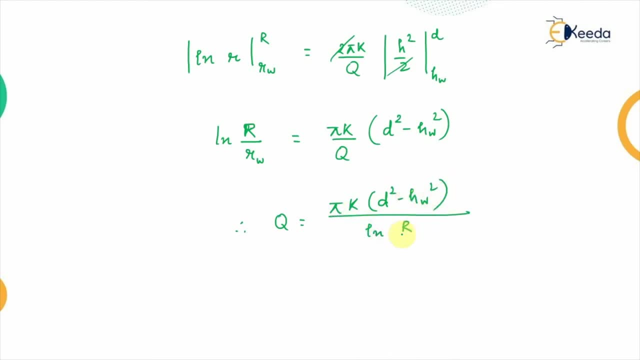 square divided by natural log of R upon rw. Now, if we remove this natural log, so this discharge can be written as pi k into d square minus hw square divided by 2 point 3 square minus hw square divided by 2 point 3 square minus hw square. Now, if we remove this natural 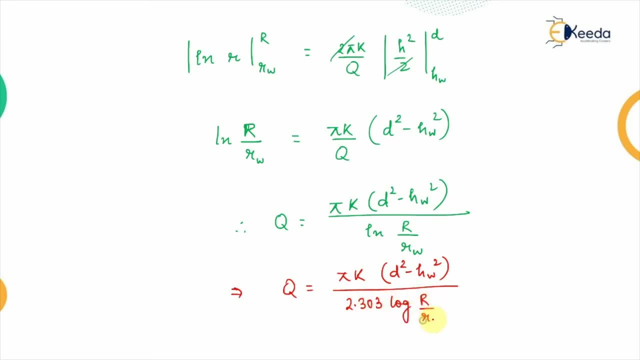 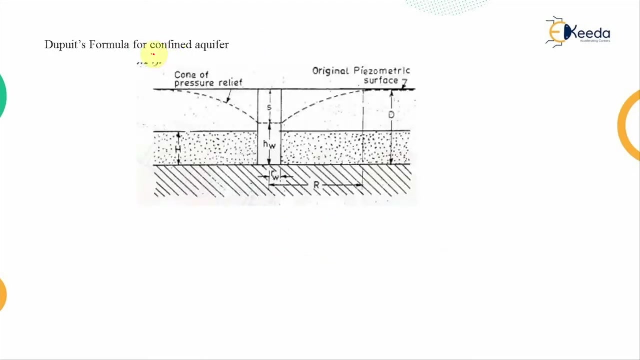 303 log base 10 R upon RW. This is the discharge through the unconfined aquifer. Now we will discuss the formula for the confined aquifer, So the Dupuyt's formula for the confined aquifer. Now, in this case you can see that both the sides are impervious and this is 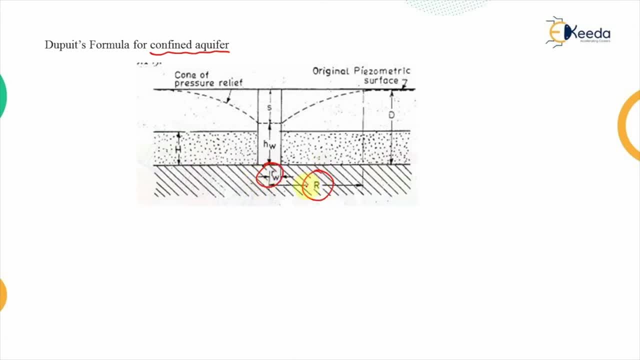 the radius RW for the main pump. well, capital, R is the radius of influence and D is the total depth, while H is the depth of the confined aquifer. Now, this is the another impervious layer. So again, we will use the same formula, that is, according to the Darcy's law, Q is 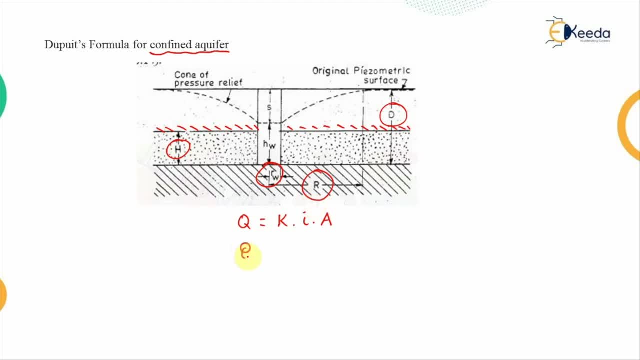 equal to K, into I, into A, Then again Q is equal to this. This K, I will be DH upon DR for smaller area, into 2 pi R up to the height H. Now this height becomes constant because always the height of water in the main well, that will be greater. 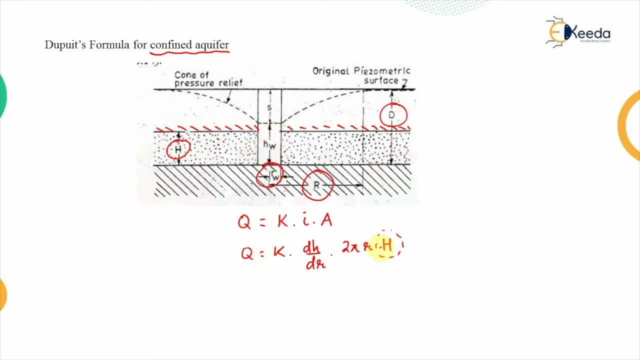 than the height of the aquifer. Therefore this will become constant. Now, if we rearrange the terms, this will be DR upon R, This is equal to 2 pi. K upon Q. Now, this time H will also be coming out, DH, Now the limits. 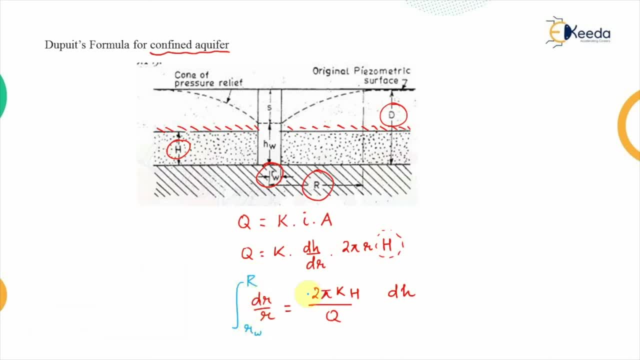 for R they are still the same, that is RW to capital R, while for DH it will be HW, that is the height of water in the main well to the total depth of the medium. that is capital D. So this is the depth of the well or height of the aquifer below the original piezometric.